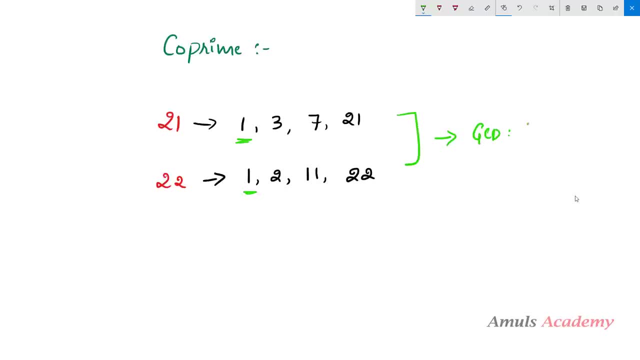 So the GCD of this is 1, so that's why this 21 and 22 are the co-prime numbers. So now, if i take another number Instead of 22,, i will take 24,, 1,, 2,, 3. ok, so these are the factors. 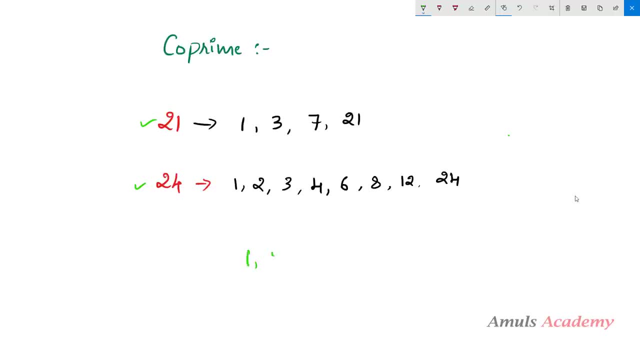 So now, if we find out the common factors: 1 is common, 3 is common, ok, 1 and 3 are common and the greatest common divisor is 3, so 21 and 22 are not co-prime- ok, because we want. 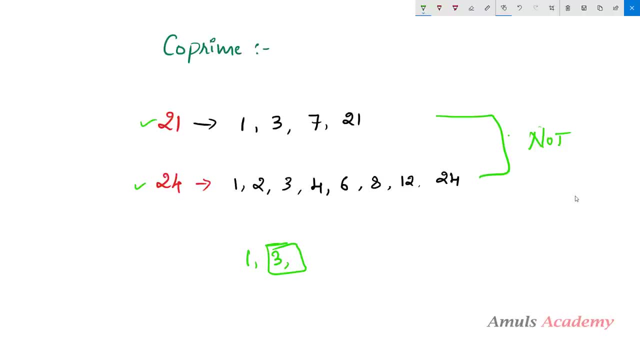 the greatest common divisor as 1,. if it is not, then they are not co-prime. So 21 and 24 are not co-prime, So don't get confused with the name. ok, it is co-prime, so don't think that two numbers. 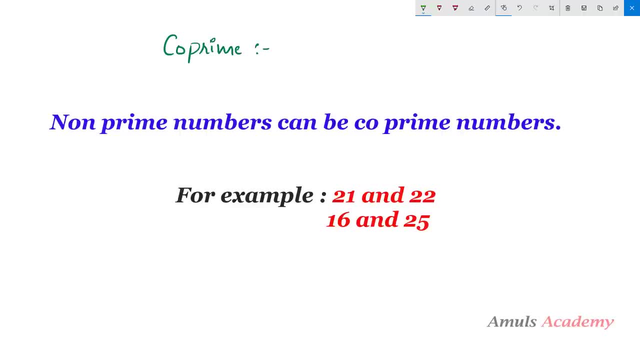 should be prime numbers. no, the non prime numbers or composite number can be co-prime. For example, if i take 16 and 25, both are co-prime. so there is no rule: like to become co-prime, it should be prime numbers. 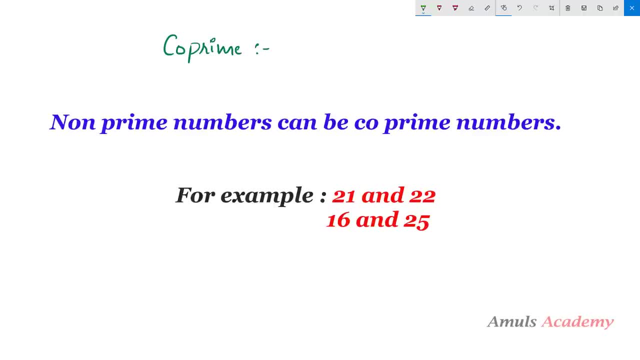 So co-prime is nothing. but if two numbers has gcd 1, or we can say greatest common divisor as 1, then that two numbers are co-primes. simple, right. So we will write the program. so this program is very simple because we just need to find: 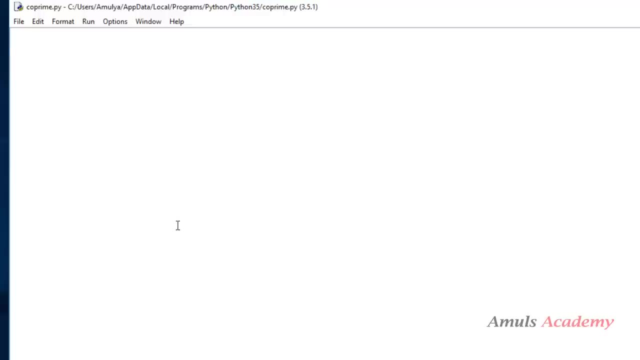 out the gcd of numbers. so here i will take two numbers, so num1,. so we want integer input. ok, So here we took the variable name as num1 and num2, so we need to take the input. this message will display on the output screen. and here we want integer input in Python. 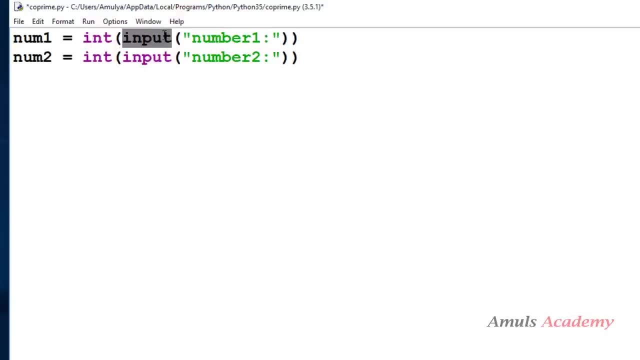 3. by default this input function will take the input. So here we took the variable name as num1 and num2, so we need to take the input. this will take input as string, but here we want integer numbers. that's why i took int function. 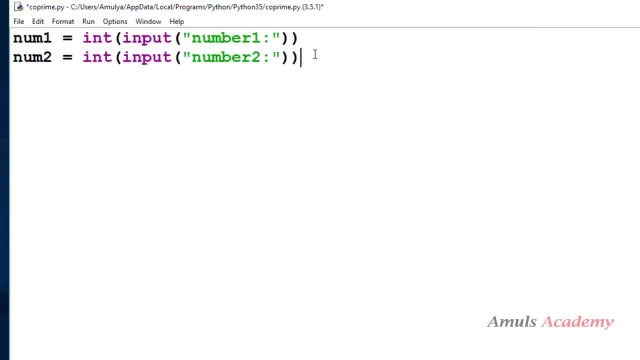 here to convert this string to integer. Alright, so we took the input. next we want to find out the gcd of this numbers. if gcd is 1, then that number is co-prime. if not, that is not co-prime, simple. 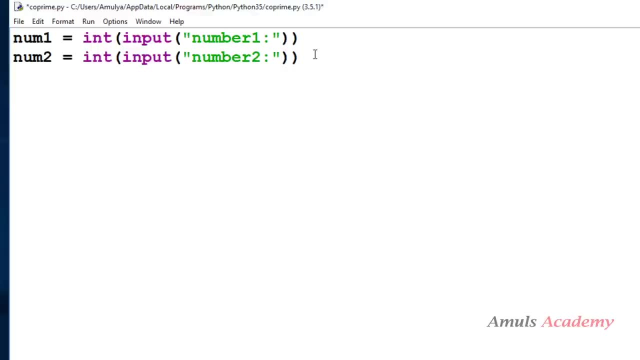 So now, how to find out the gcd so we can define the gcd function using the Euclid's algorithm. We already discussed about this And i already uploaded a video on this, so i will give you the link in the description box. go and check that, ok. 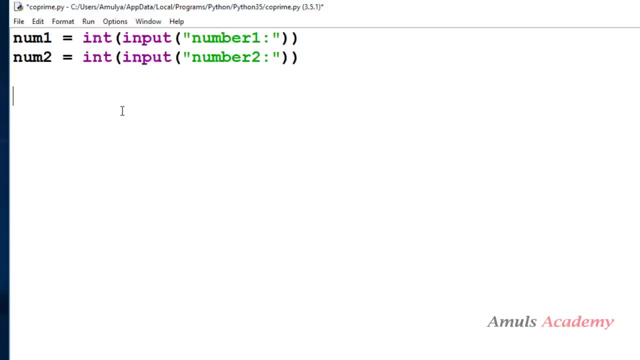 So you can define gcd function here and you can call that function to find out the gcd of two numbers. Or i can use the gcd function which is already defined in fractions library, So i can just import that library and i can use the gcd function. 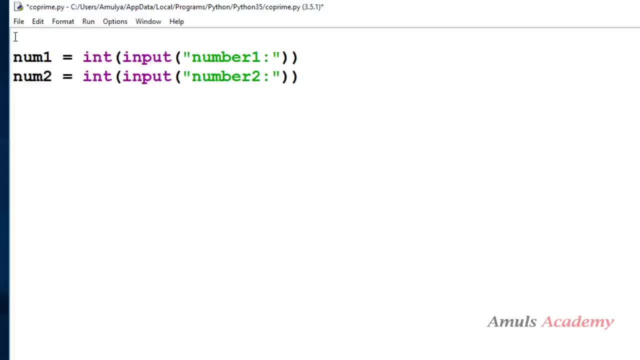 Here i am doing that. i am not defining the gcd function here. If you want to define the gcd function, go to the description box and click on that video link and watch that video and you can define the gcd function. So here i will: import from fractions, import gcd- ok, i want gcd function. so from fractions. 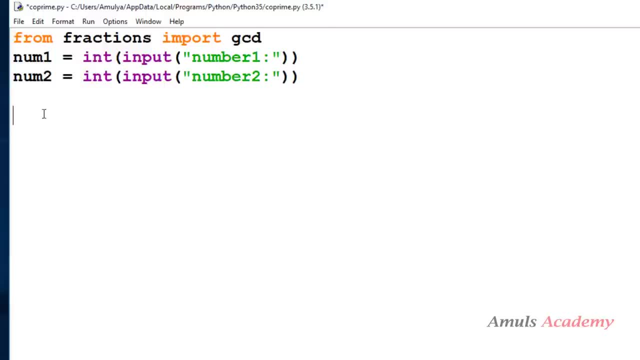 library import gcd. Next, here i will just take if gcd of num1 and num2.. Ok, So we have done that. So here i will just take if gcd of num1 and num2.. num2 is equal to equal to 1, print given numbers are co prime, or you can take num1. 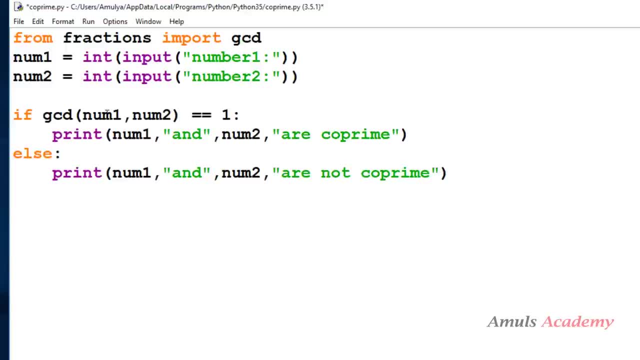 So i will check the gcd of num1 and num2. i will use the built in function. So if it is 1 of num1 and num2, so these numbers are co prime. if not, it is not co prime. So i will execute this. 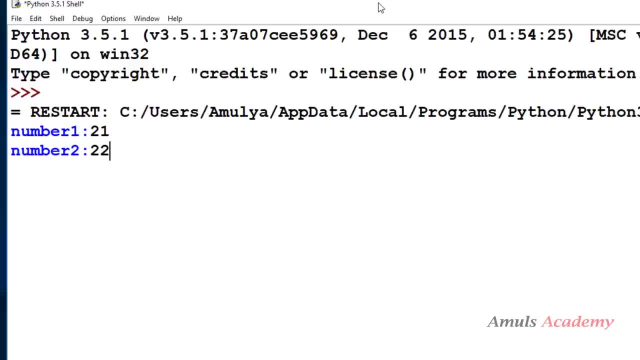 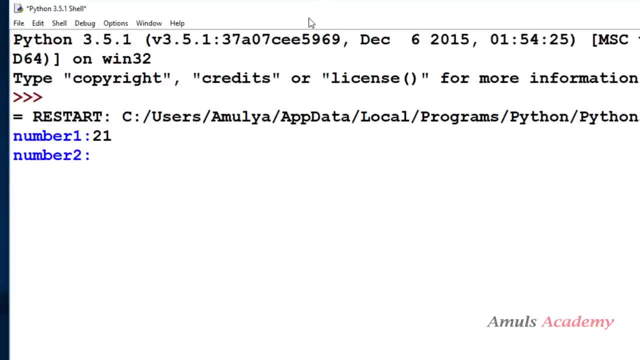 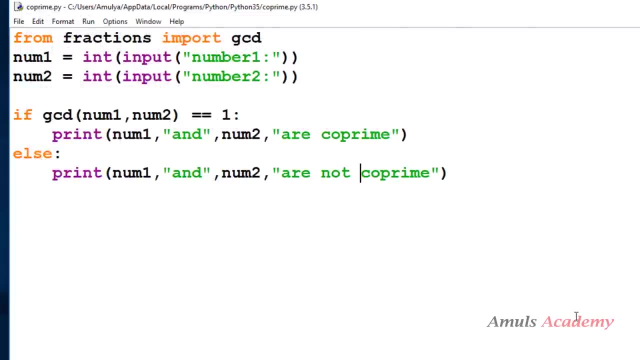 So number 1, so i will enter 21,, 22,, 21 and 22 are co prime true, right. i will enter 21 and 24 are not co prime true, right? Ok, Ok. So this is about this co prime program.